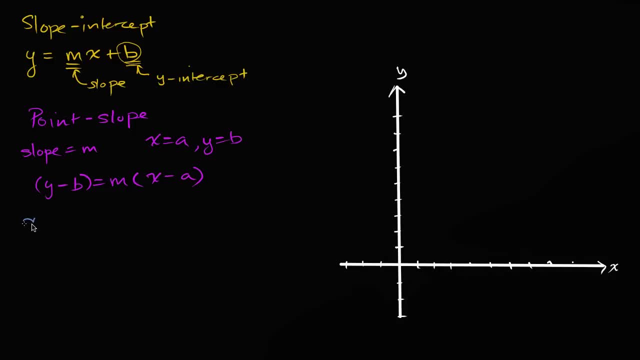 that you might have already seen, And that is standard form, Standard, standard form. And standard form takes the shape of ax plus b. y is equal to c, where a, b and c are integers. And what I want to do in this video. 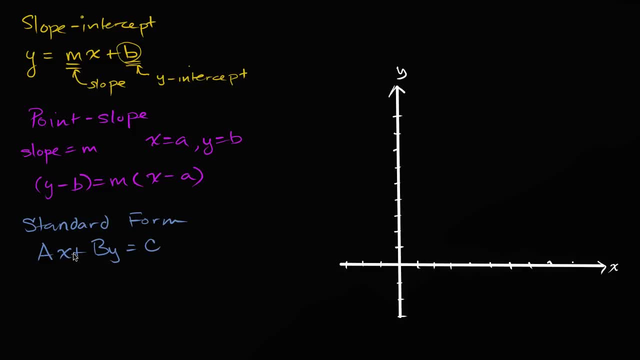 like we've done in the ones on point-slope and slope-intercept, is gain an appreciation for what is standard form good at and what is standard form less good at. So let's give a tangible example here. So let's say I have the linear equation. 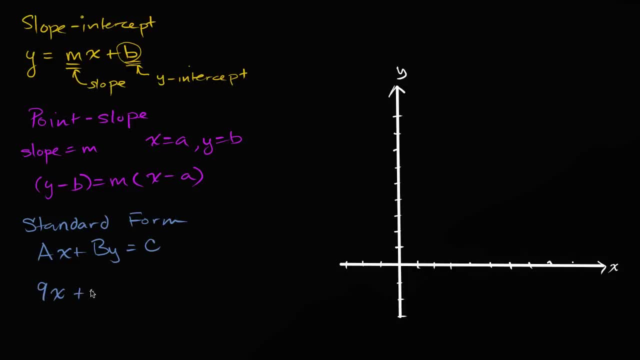 It's in standard form: Nine x plus 16y is equal to 72. And we want to know and we wanted to graph this. So the thing that standard form is really good for is figuring out not just the y-intercept. 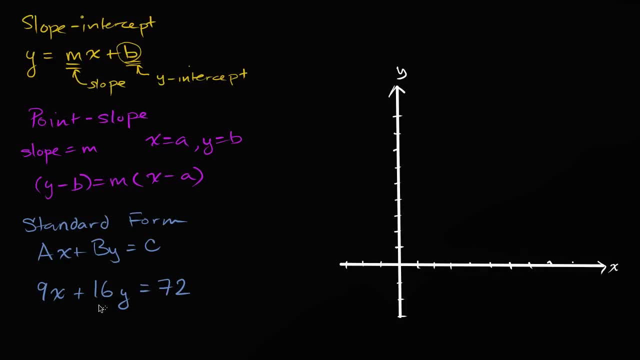 y-intercept is pretty good if you're using slope-intercept form, but we can figure out the y-intercept pretty clearly from standard form and the x-intercept. The x-intercept isn't so easy to figure out from these other forms right over here. 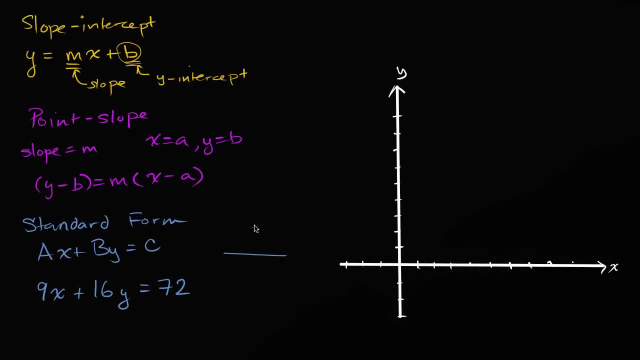 So how do we do that? Well, to figure out the x and y-intercepts, let's just set up a little table here: X comma y, And so the x-intercept is going to happen when y is equal to zero. 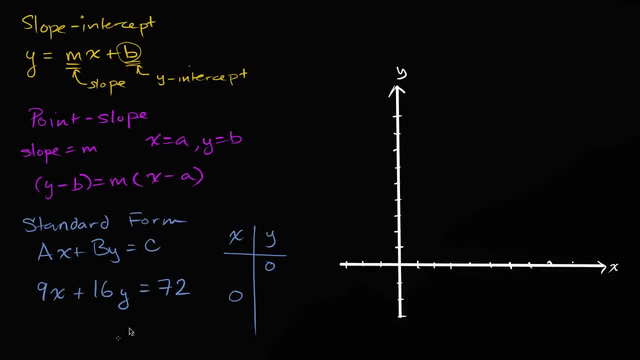 and the y-intercept is going to happen when x is equal to zero. So when y is zero, what is x? So, when y is zero 16 times zero is zero, that term disappears and you're left with nine. x is equal to 72.. 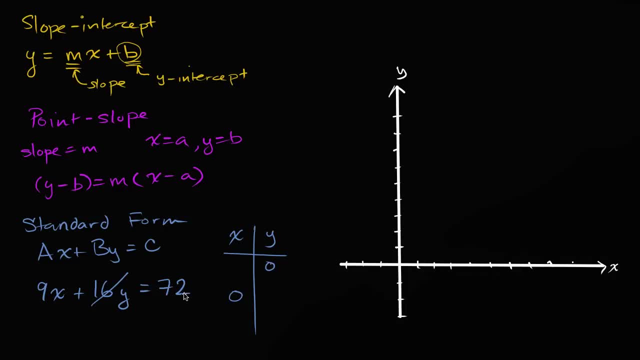 So if nine times x is 72,, 72 divided by nine is eight. So x would be equal to eight. So once again, that was pretty easy to figure out. This term goes away and you just have to say: hey, nine times x is 72,, x would be eight. 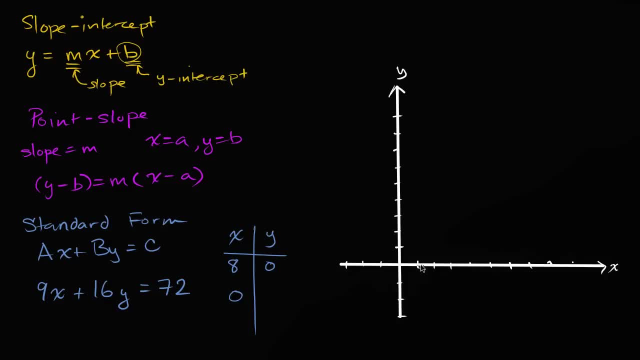 When y is equal to zero, x is eight. So the point let's see: y is zero, x is one, two, three, four, five, six, seven, eight. that's this point, That right over here, this point, right over here. 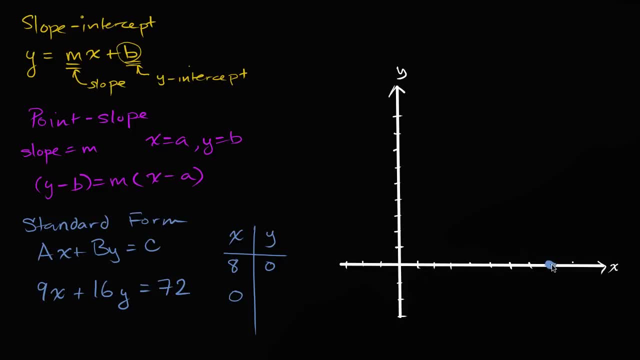 is the x-intercept. When we talk about x-intercept, we're referring to the point where the line actually intersects the x-axis. Now, what about the y-intercept? Well, we set x equals zero. This disappears and we're left with 16y is equal to 72.. 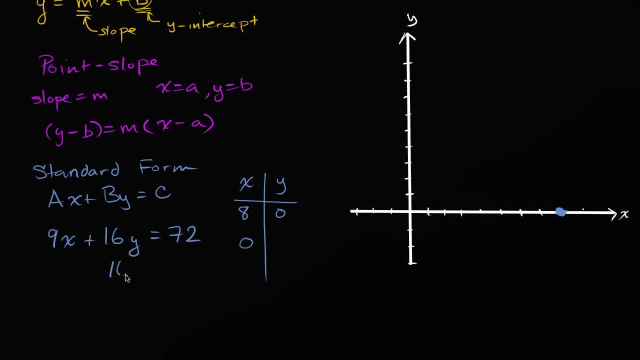 And so we could solve. we could solve that. So we could say: all right, 16y is equal to 72, and then divide both sides by 16, we get y is equal to 72 over 16, and let's see what is that equal to. 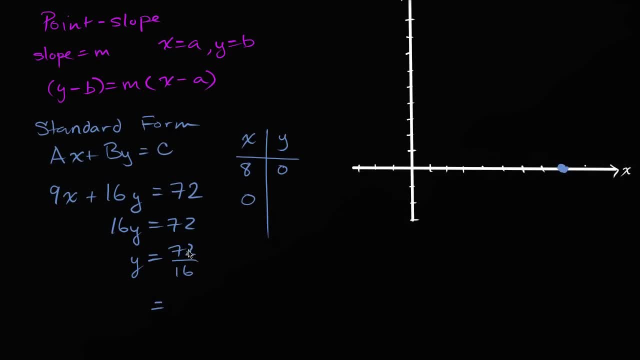 That is equal to. let's see, they're both divisible by eight, So that's nine over two. or we could say it's 4.5.. So when x is zero, y is 4.5. And so we could plot that point as well. 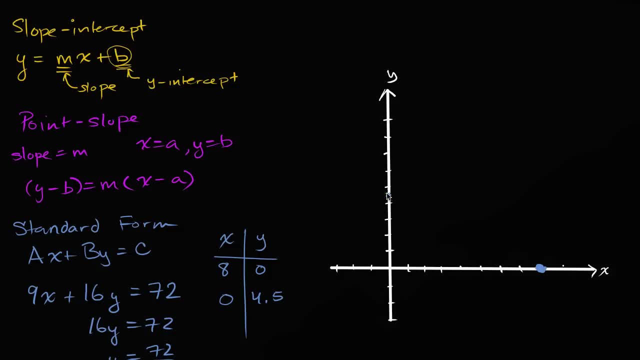 X is zero, y is one, two, three, four, .5.. And just with these two points. two points are enough to graph a line. we can now graph it. So let's do that. So let me. whoops, I thought I was using the tool. 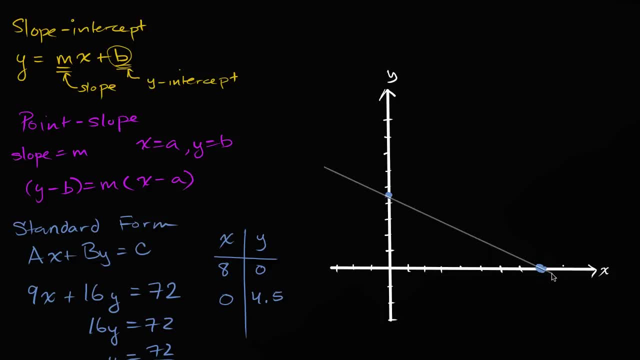 that would draw a straight line. Let me see if I can. so the line will look something like that. There you have it. I've just graphed. I've just graphed. this is the line that represents all the x and y pairs. 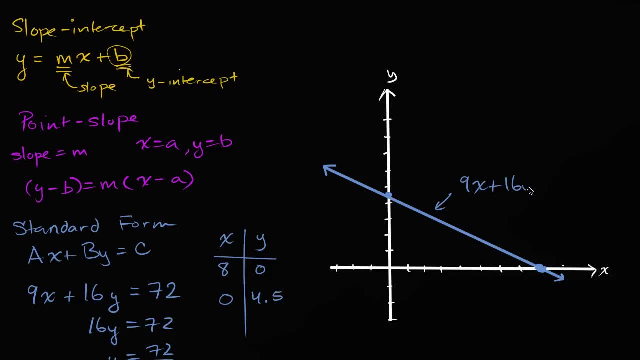 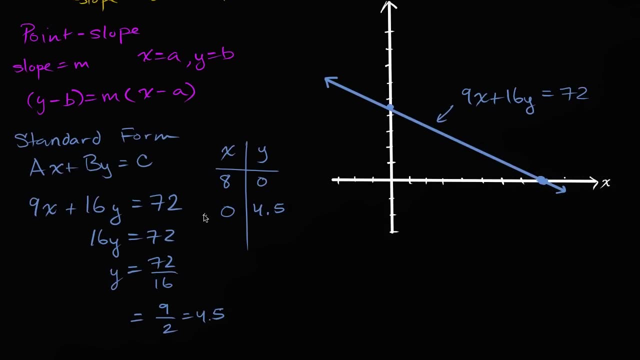 that satisfy the equation. nine x plus 16y is equal to 72.. Now I mentioned standard form's good at certain things and the good thing that standard form is where it's maybe somewhat unique relative to the other forms we looked at. 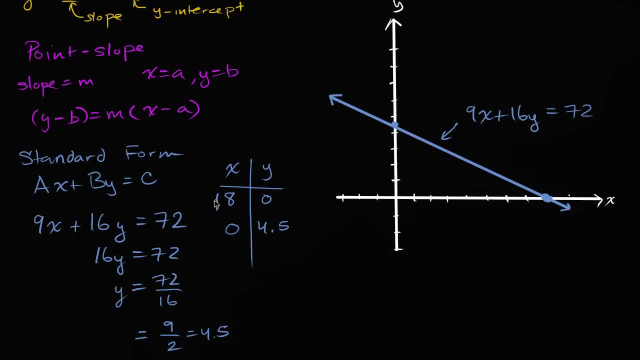 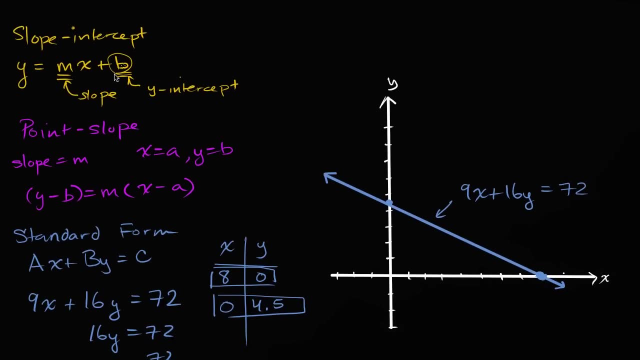 is. it's very easy to figure out the x-intercept. it was very easy to figure out the x-intercept from standard form and it wasn't too hard to figure out the y-intercept either If we looked at slope-intercept form. 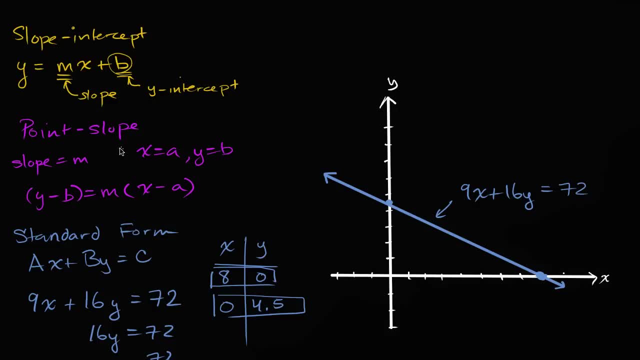 the y-intercept just kind of jumps out at you. At point-slope form, neither the x nor the y-intercept kind of jump out at you. The place where slope-intercept or point-slope form are frankly better is that it's pretty easy. 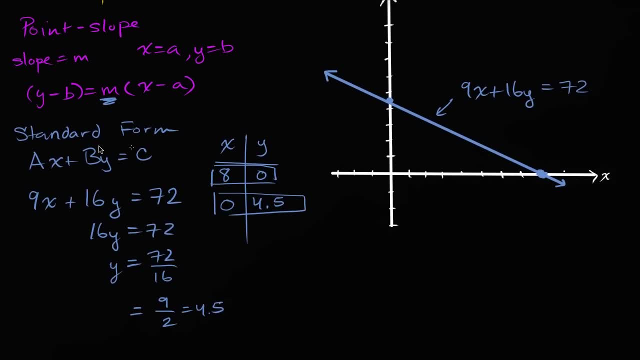 to pick out the slope here, while in standard form you would have to do a little bit of work. You could use these two points. you could use the x and y-intercept as two points and figure out the slope from there. so you could literally say: 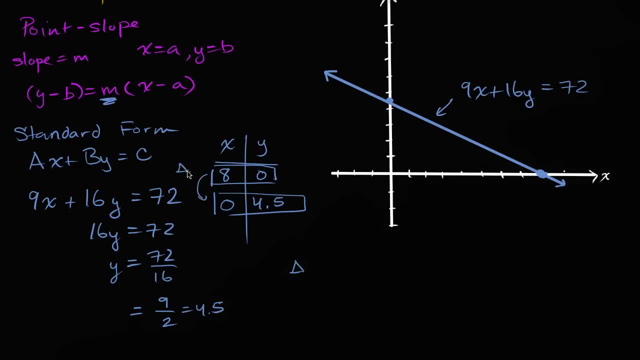 okay, if I'm going from this point to this point, my change in x to go from eight to zero is negative eight and to go from zero to 4.5, or the little delta there unnecessarily. let me so when you go from eight to zero. 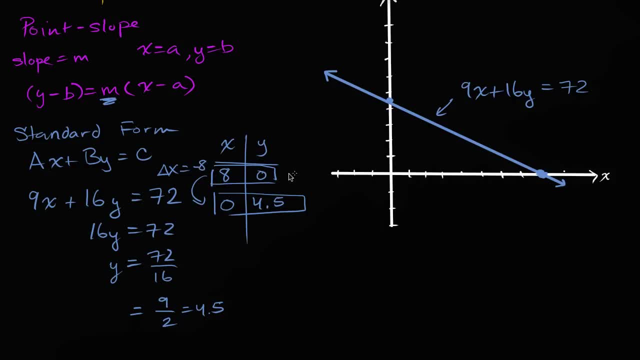 your change in x is equal to negative eight, and to go from zero to 4.5,, your change in y is going to be 4.5, so your slope. once you've figured this out, you could say: okay, this is going to be. 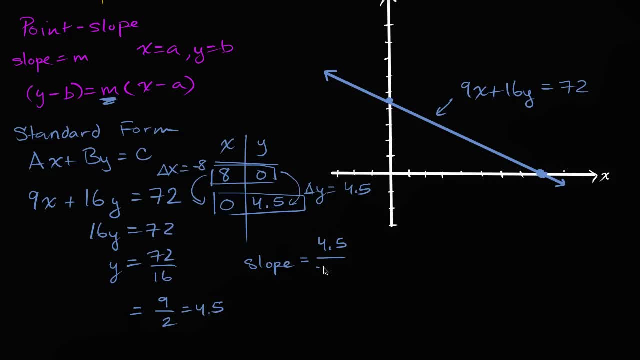 change in y 4.5, over change in x over negative eight. and since at least I don't like a decimal up here, let's multiply the numerator and the denominator by two. you get negative nine over 16.. 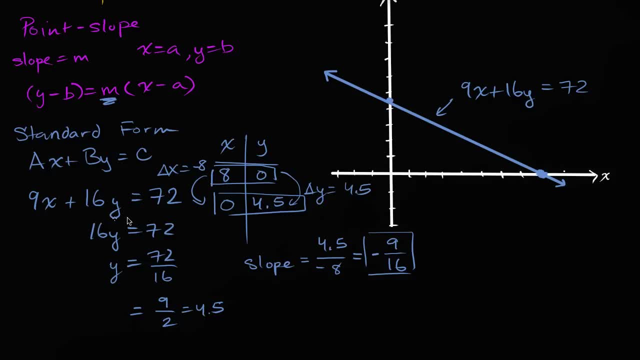 Now, once again, we have to do a little bit of work here. We either use these two points- it didn't just jump immediately out of this, although you might see a little bit of a pattern of what's going on here, but you still have to think about. 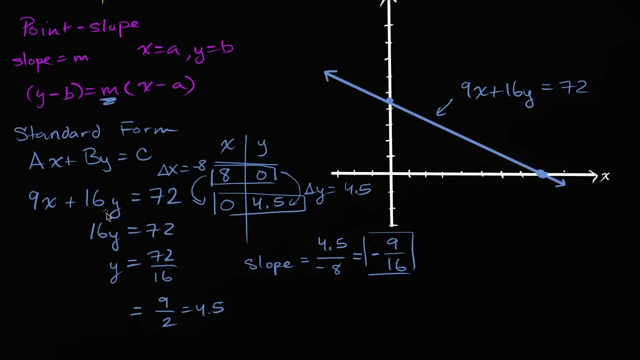 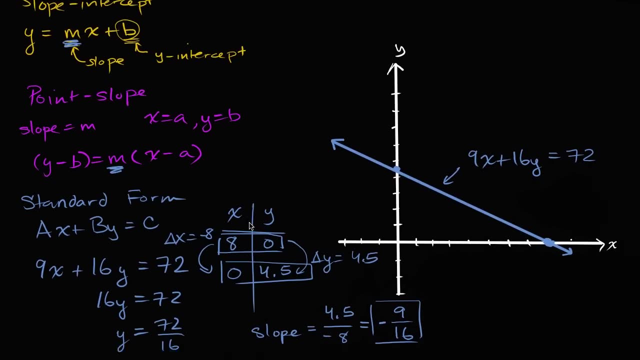 is it negative? is it positive? You have to do a little bit of algebraic manipulation, or what I typically do. if I'm looking for the slope, I actually might put this into one of the other forms, especially slope-intercept form. 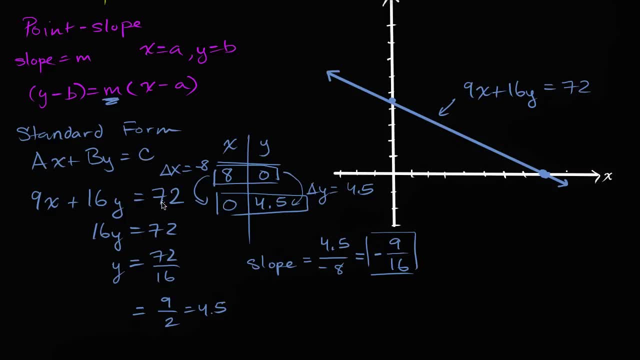 but standard form by itself, great for figuring out both the x and y intercepts, and it's frankly not that hard to convert it to slope-intercept form. Let's do that just to make it clear. So if you start with nine x, 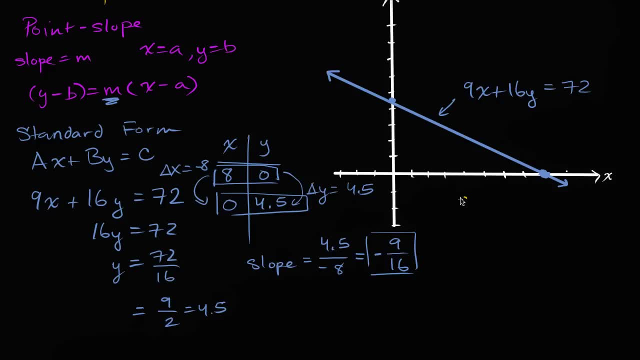 let me do that in yellow. If we start with, nine x plus 16y is equal to 72, and we want to put it in slope-intercept form. we can subtract nine x from both sides. you get 16y is equal to negative nine x plus 72,. 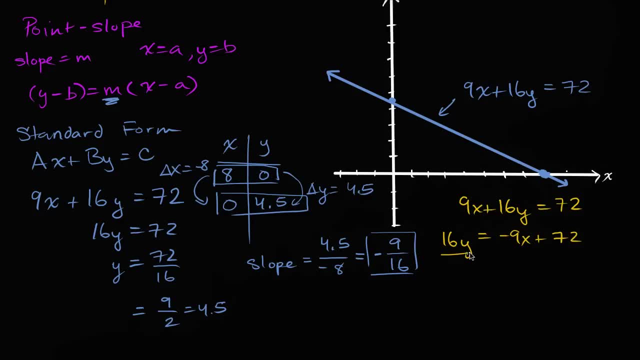 and then divide both sides by 16.. So divide everything by 16, and you'll be left with. y is equal to negative nine 16x. that's the slope. you see it right there, plus 72 over 16,. we already figured out. 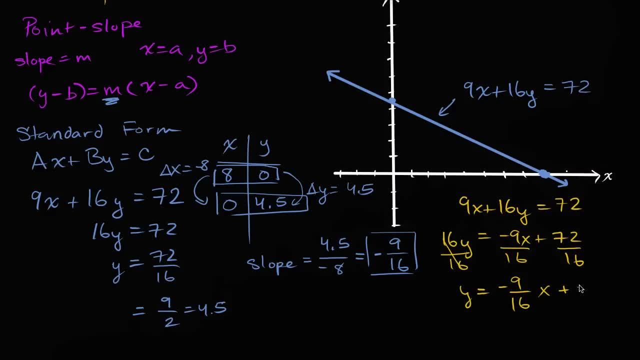 that's nine halves or 4.5. So I could write: well, I'll just write that as 4.5. And this form over here much easier to figure out. the slope and actually the y-intercept jumps out at you. but the x-intercept isn't as obvious.